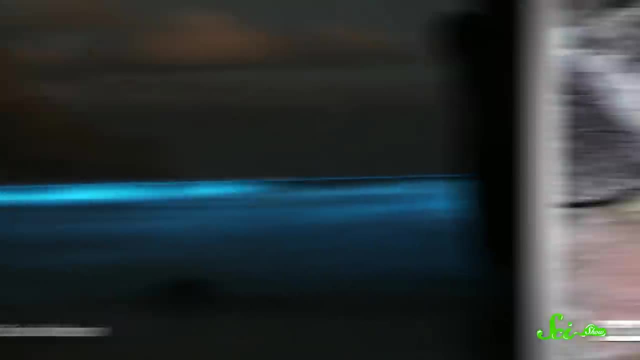 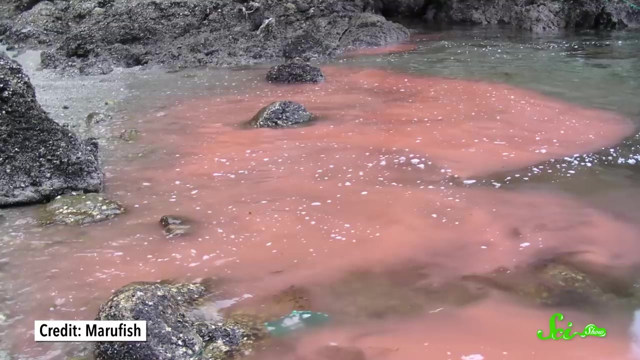 own light, Which makes for some really magical effects, But too many of them in one place can create a harmful algal bloom- a phenomenon you might have heard referred to as red tide, Which is just one example of how these super-teeny creatures can have a big impact on the rest. 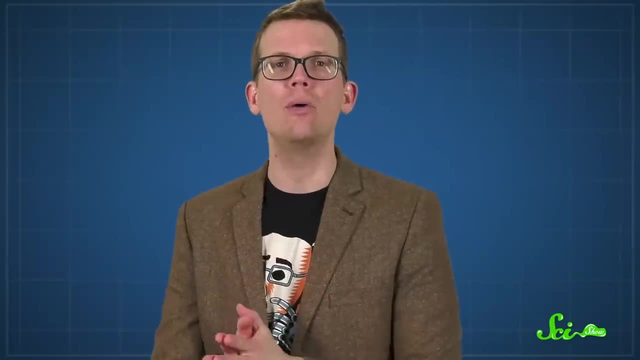 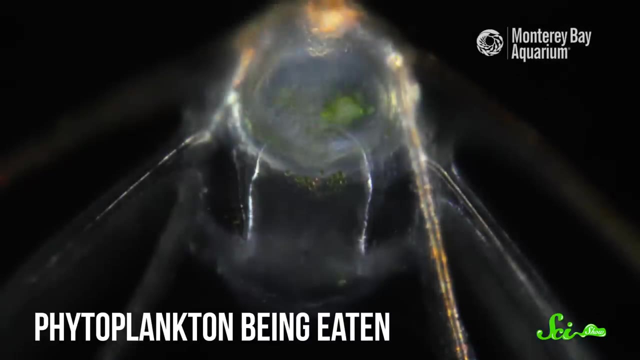 of us, even us landlubbers. No matter what form phytoplankton take, they are unbelievably important to all life on Earth. First off, they're the foundation of the marine food web, underpinning everything for us, from anchovies to whales. In fact, with a wee bit of help from seaweed and aquatic plants, they manage to support life in the ocean, despite being outweighed by roughly 5 to 1 by organisms that don't make their own food. And if that's not enough, they are also atmosphere-altering machines. 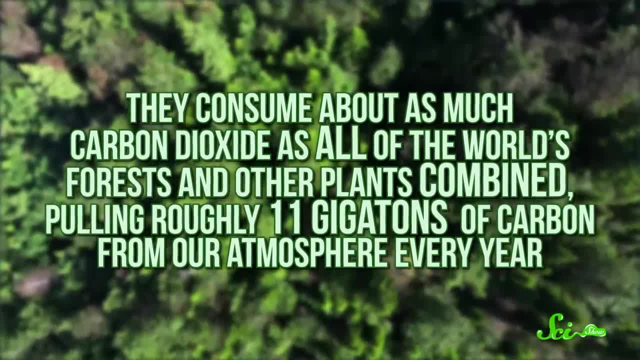 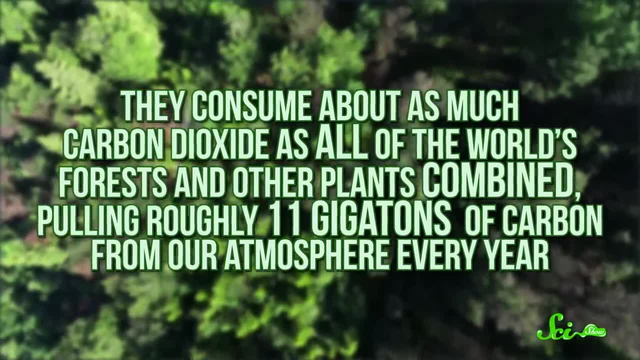 They consume about as much carbon dioxide as all of the world's forests and other plants combined, pulling roughly 11 gigatons of carbon from our atmosphere every year, Which is especially impressive when you consider that, by mass, there's about 450 times. 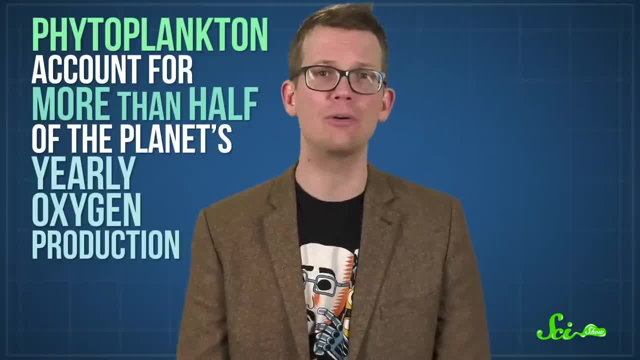 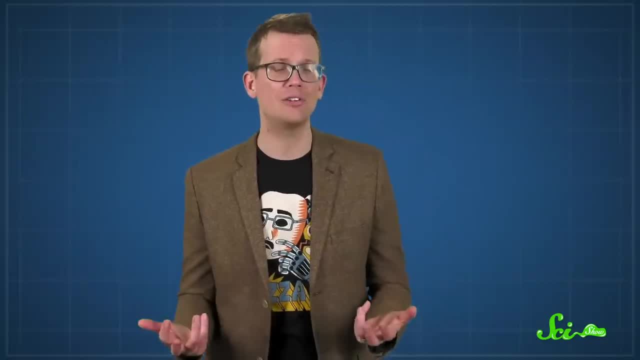 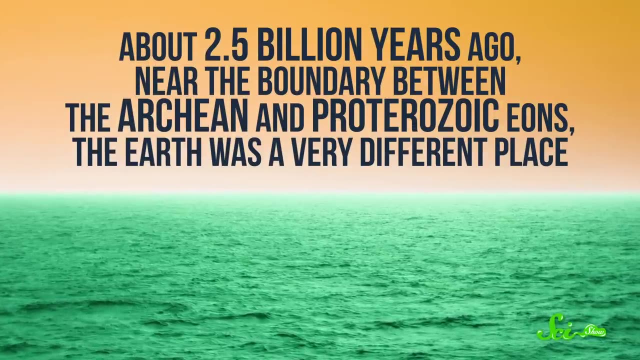 as much plant life on land Plus phytoplankton, account for more than half of the planet's yearly oxygen production. But even more importantly, they're kind of the reason we have oxygen in the atmosphere at all, Back about 2.5 billion years ago, near the boundary between the Archean and Proterozoic. 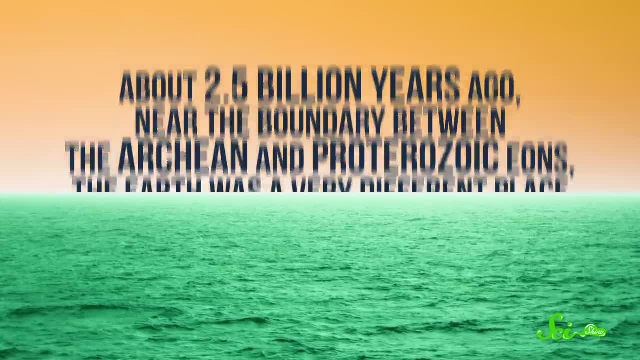 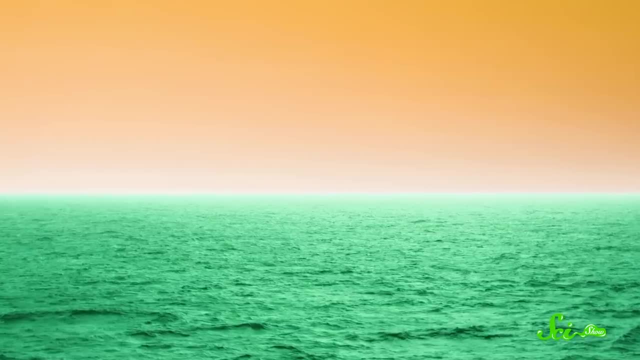 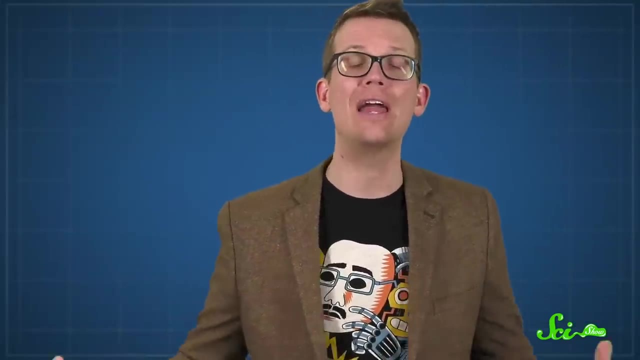 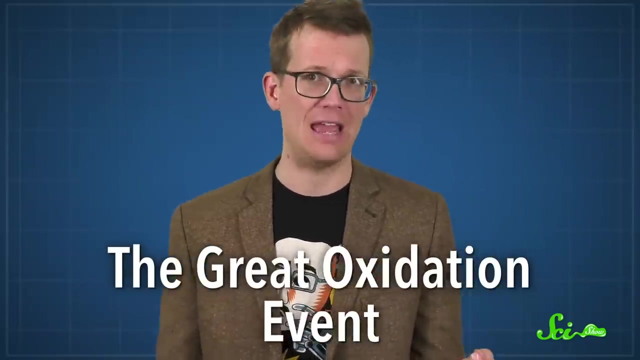 There were green skies and the atmosphere was likely a mix of gases like ammonia and methane that would immediately kill us. Then cyanobacteria evolved and ran rampant, pumping out a huge amount of oxygen in what's now called the Great Oxidation Event. 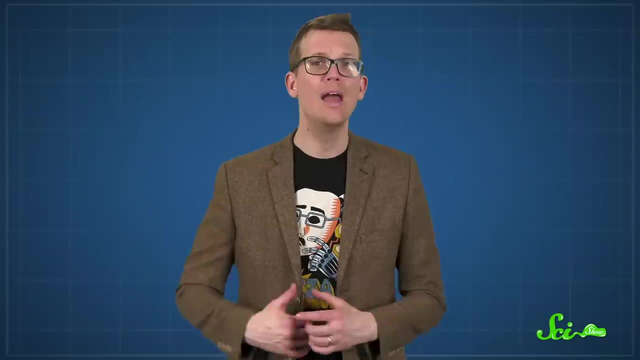 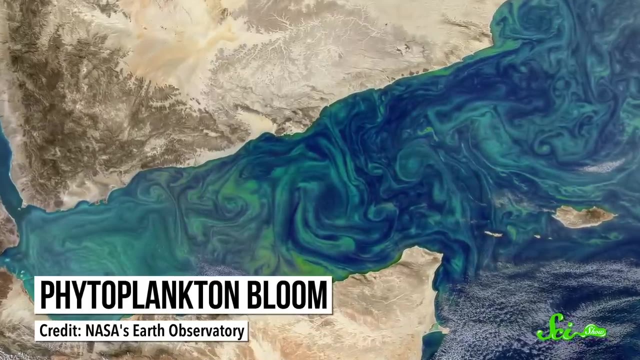 All that oxygen helped turn the ocean and skies blue and likely jump-started the evolution of complex life. And then, around 540 million years ago, phytoplankton did it again, exploding in numbers and bringing us up to more or less the levels of oxygen in the atmosphere we 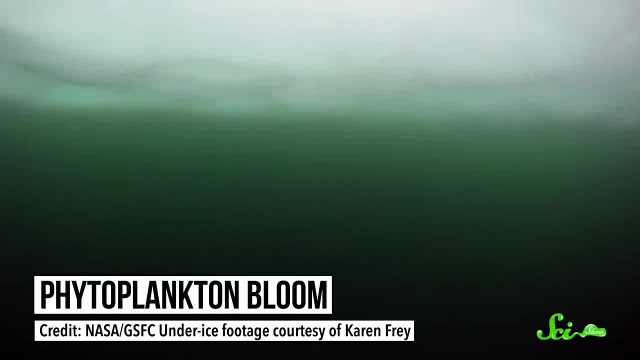 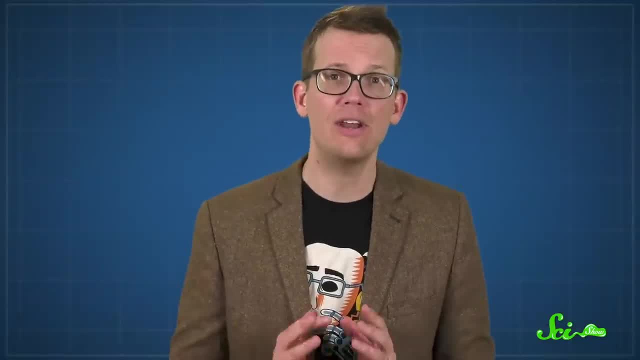 have today. Paleontologists think the boom may have occurred thanks to nutrients weathered out of rocks by giant continent-sized glaciers. Or a more recent idea is that it happened because the plankton evolved a more efficient internal machinery related to photosynthesis. 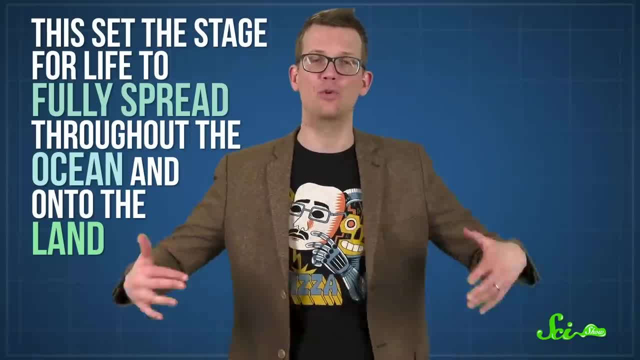 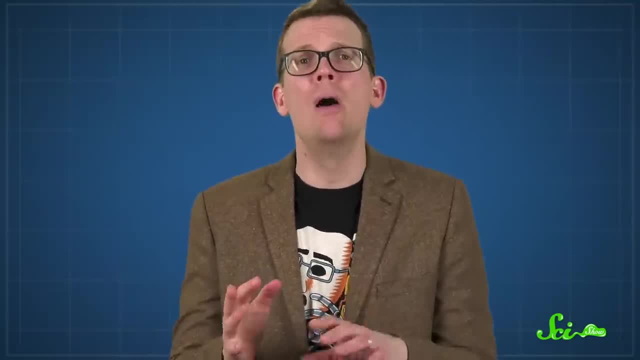 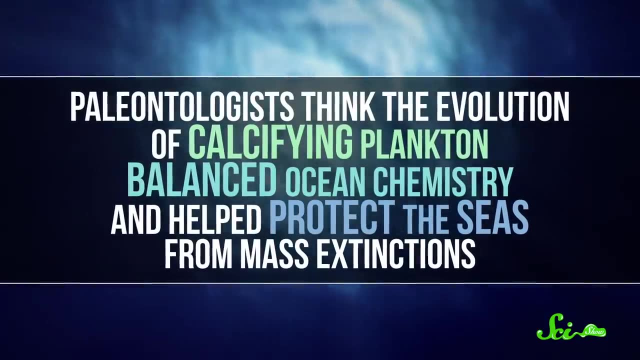 Either way, this set the stage for life to fully spread throughout the ocean and onto the land. Since then they've calmed down on reshaping the entire planet front And adopted more of a stabilizing role. For example, paleontologists think the evolution of calcifying plankton balanced ocean chemistry. 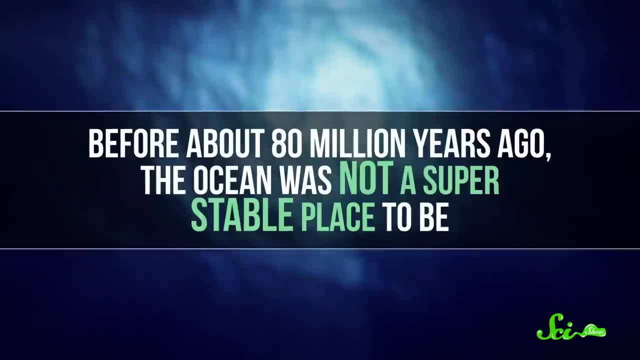 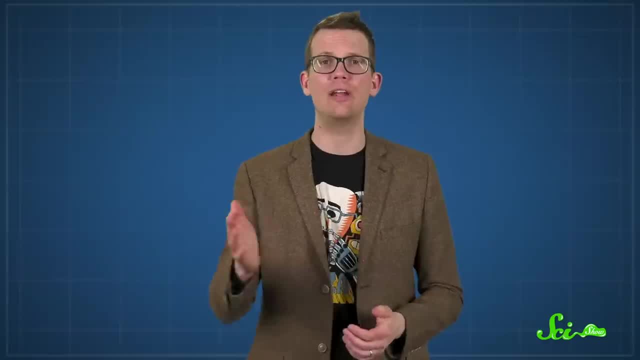 and helped protect the seas from mass extinctions. Before about 80 million years ago, the ocean was not a super-stable place to be. Changes in the chemistry of the atmosphere from events like volcanic eruptions often caused deadly swings in seawater pH. 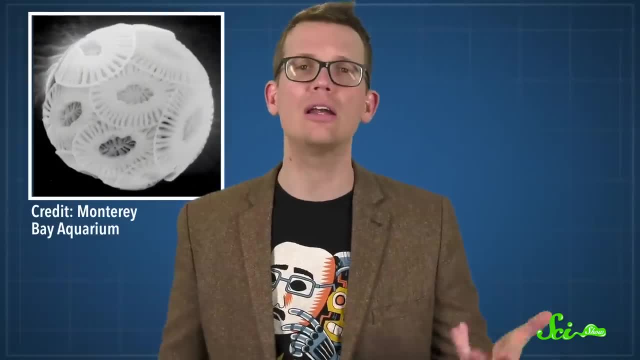 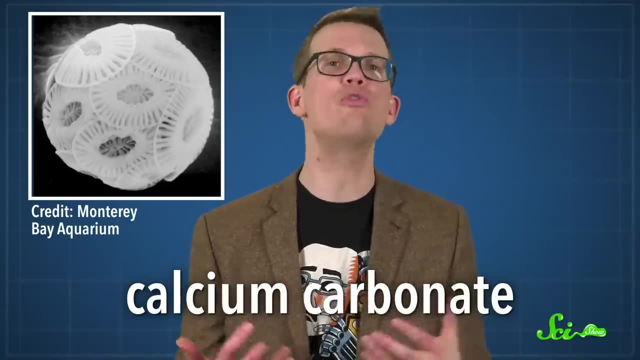 Then some lineages of plankton—including those ball-like coccolithophores—figured out as a result that the ocean was not a stable place to be. So they figured out how to make shells of calcium carbonate. Soon they took over the open ocean. 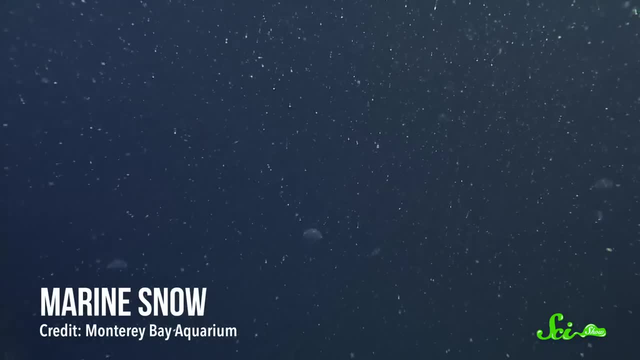 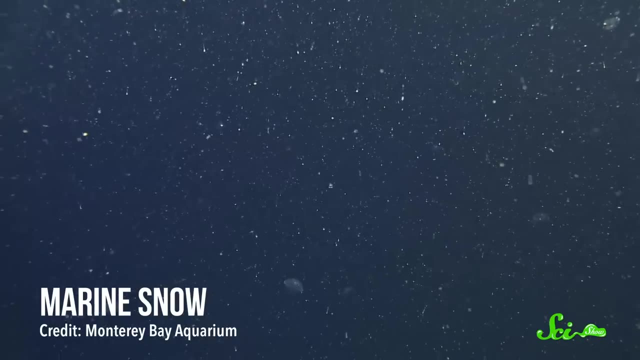 And over a relatively short period of time. so many of their shells sank to the depths of the oceans that they created a vast, thick layer of calcium carbonate ooze on the seafloor. That ooze acts as a chemical buffer in the ocean—a natural breaking system on runaway. 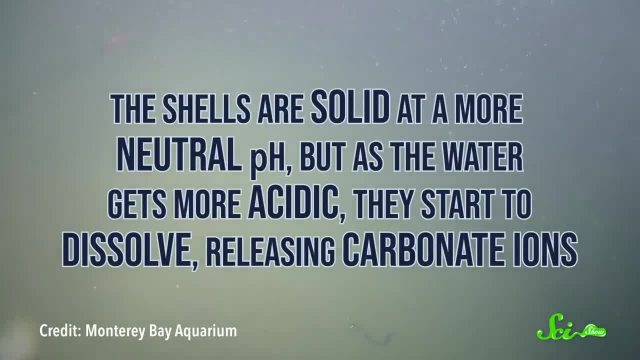 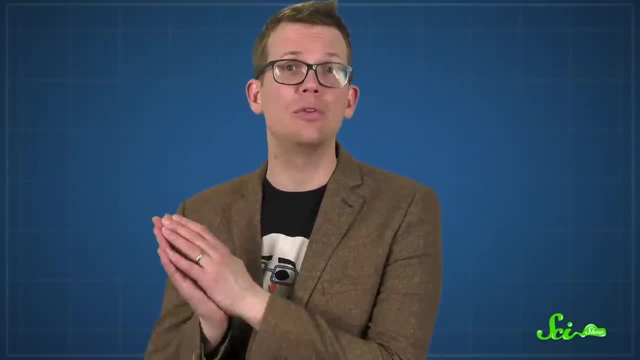 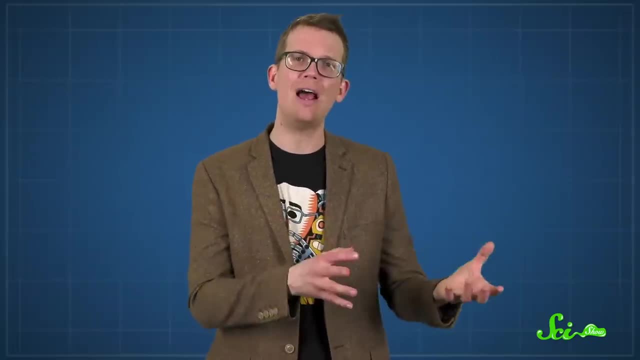 acidity. See, the shells are solid at a more neutral pH, but as the water gets more acidic they start to dissolve, releasing carbonate ions Those chemically react with the surrounding seawater to push an acidic pH back towards neutral. Now there had been a minor version of this in the shallows, thanks to mollusks and other. 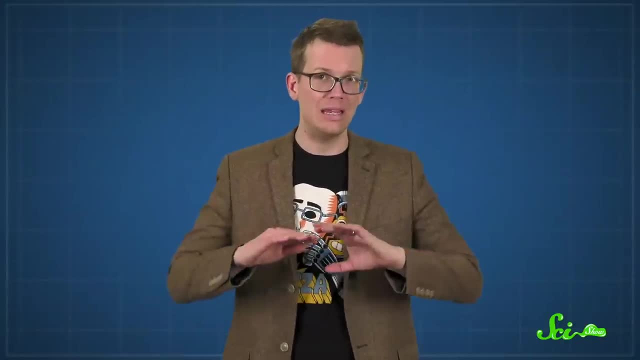 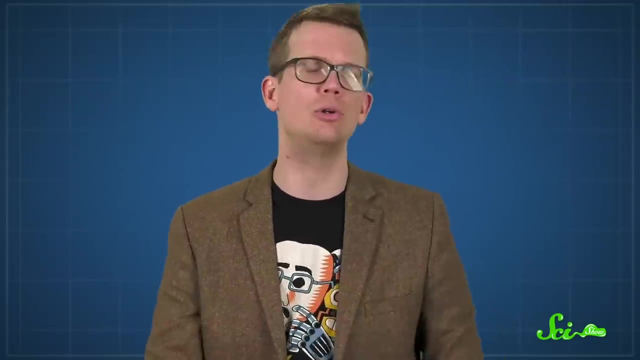 large shelled organisms, but it took phytoplankton to make it ocean-wide, And the end result was a more stable ocean chemistry, which meant marine life became less vulnerable to things like volcanic eruptions. Even today, this chalk layer is helping buffer the acidifying effects of calcium carbonate. 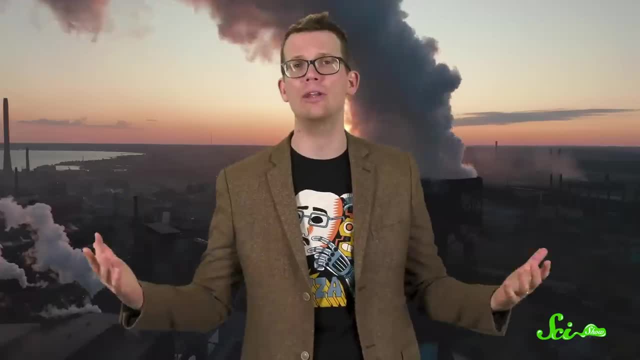 But it's not enough. It's not enough. It's not enough. Life is more beautiful when it's not. It's not enough to know the acidifying effects of all the carbon dioxide that we humans are pumping into the atmosphere. Though there's only so much it can do. When we consider everything that lives in the ocean, from majestic whales to bountiful coral reefs, these little unassuming phytoplankton are easy to overlook, But if you look at the history of Earth, it doesn't take long to realize that though. 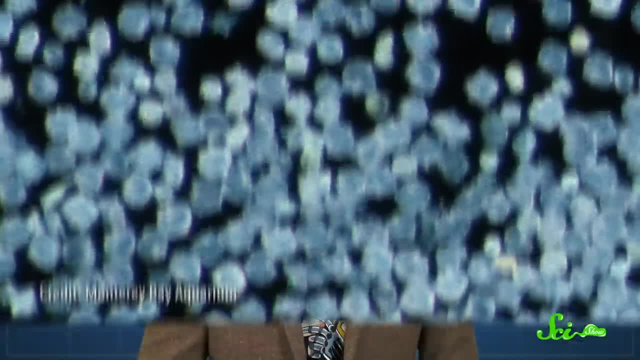 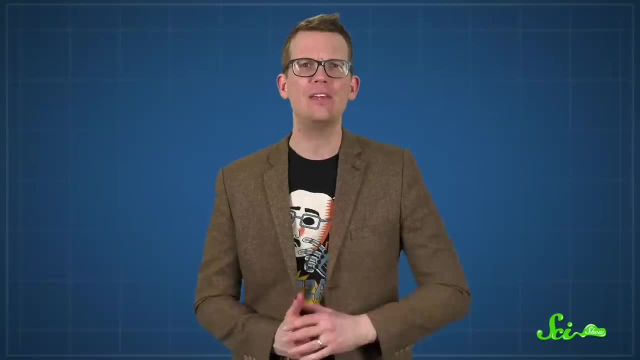 they are small, they are also mighty And they deserve as much fascination, love and protection as any other planet. But if you look at the history of the planet, you're not going to get that question. the one after the other other living thing on this planet.